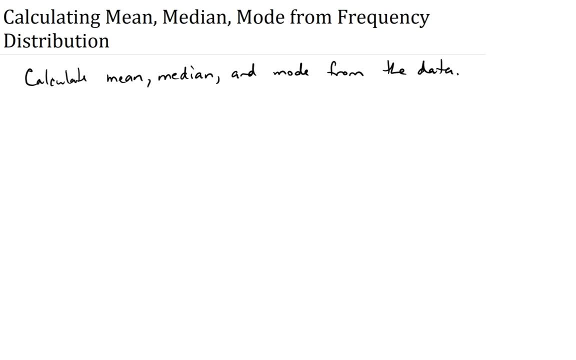 From the data. So let me give you some data. This is what we call a frequency distribution. Whenever you have data values that repeat, then you might want to list them in a frequency distribution. So let's, we'll have a column for our data. 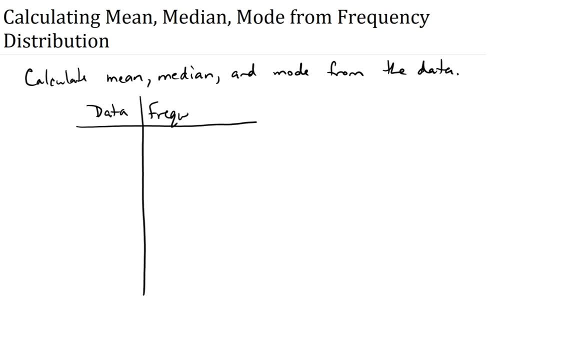 We'll have a column for our frequency, Okay, so let's say we'll kind of keep it simple here. Let's say we have five data values. Let's say we have 70, 80, 90, 100, 110.. 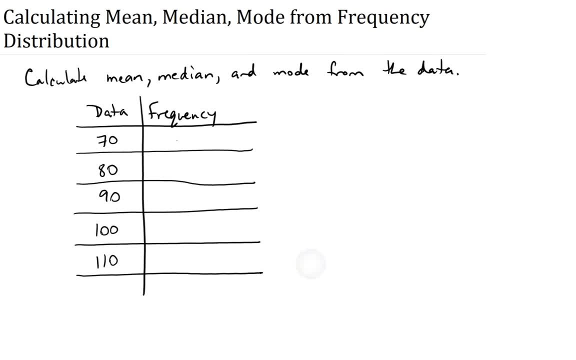 And then we have frequencies for these. I'll talk about what that means. Let's say, I have 5, 10,, 11, 8.. Okay, all this means is these are your data values, and frequency is how many times each occurs. 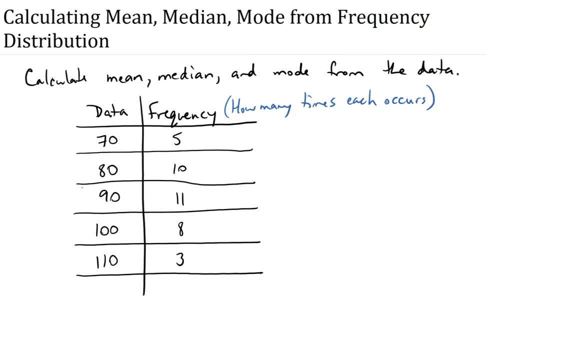 Okay. So if I were to list, if I were simply to list this data, it would look like this And put it in order. let's say I'd have a 70, and then I'd have 100.. 1,, 2,, 3,, 4 more 70s. 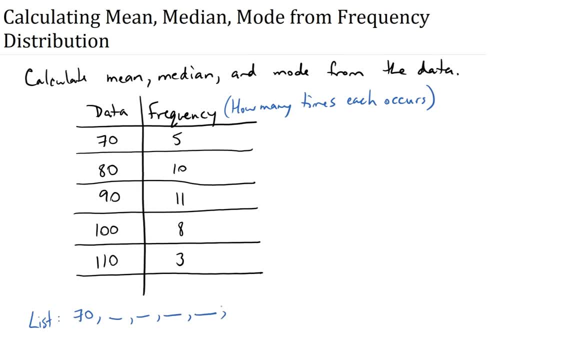 So that would be 5- 70s. I'm just not going to write them all out. That's the whole point of the frequency distribution. So this up here, let me tell you that It's called frequency distribution. Okay, Then I'd have 10,, 80. 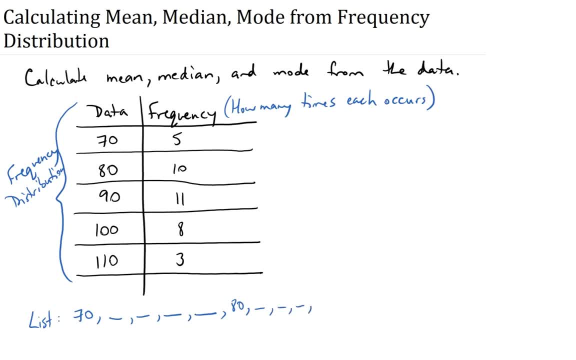 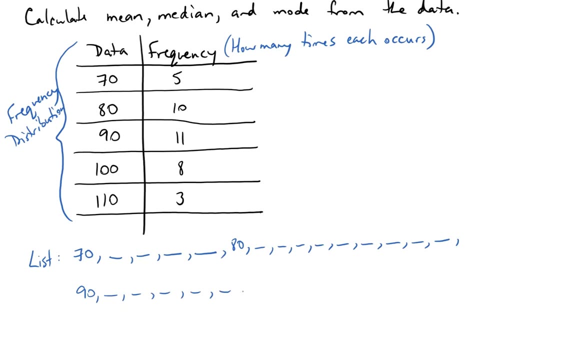 So I'd have an 80, and I'd have 9 more. You can see why you don't want to list all of these out. Then I'd have 11- 90s. Let's see 1,, 2,, 3,, 4,, 5,, 6,, 7,, 8,, 9,, 10,, 11 90s. 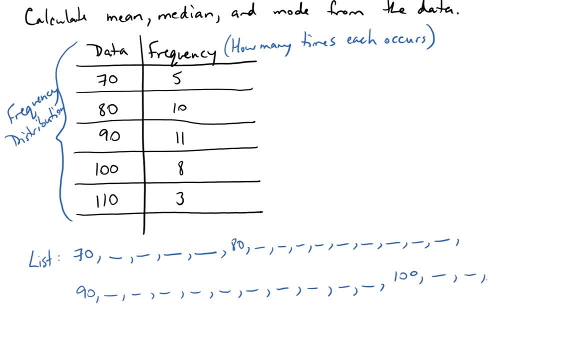 I'd have 8 100s, Then I'd have 3 110s, which I could certainly list out. Maybe There we go. So that would be our list of data in order. So if I want the mean, for example, 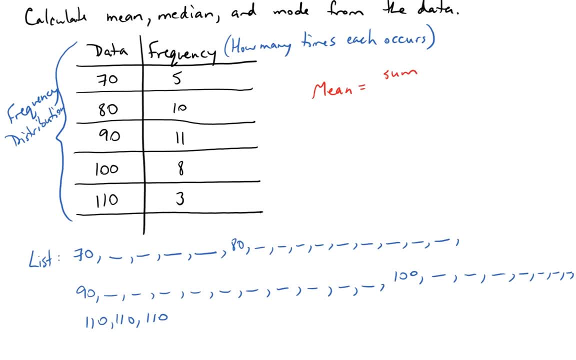 The mean would be the sum of all those. Add them all up Divided by how many there are. Okay, Now I could use my list to do that, But that would be absurd, right? Why would I want to add 5 70s and 10 80s? 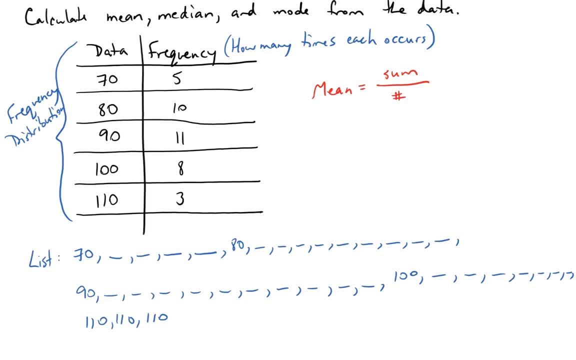 11. 11, 90s, et cetera. So my sum is simply going to be: Well, 5- 70s is precisely 70 times 5.. Then I've got 10- 80s, so that's 80 times 10.. 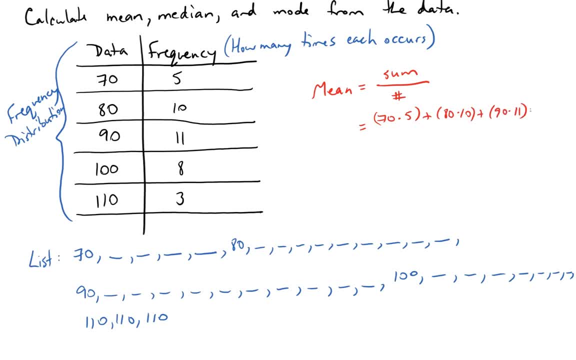 And then 90, 11 times, And then 100, 8 times- Let's move this over a little bit- And finally 110, 3 times. That would be my sum, And then I would divide by how many data values there are. 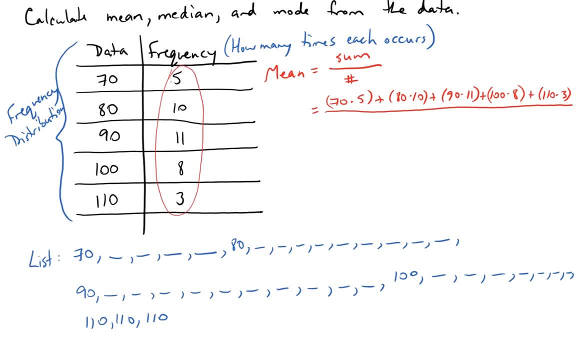 I could certainly count them, or I could just add my frequencies. Okay, If I add my frequencies, then I'd have 15,, 26,, 34,, 37 data values And you could calculate that rather quickly, And I hope I did this right. 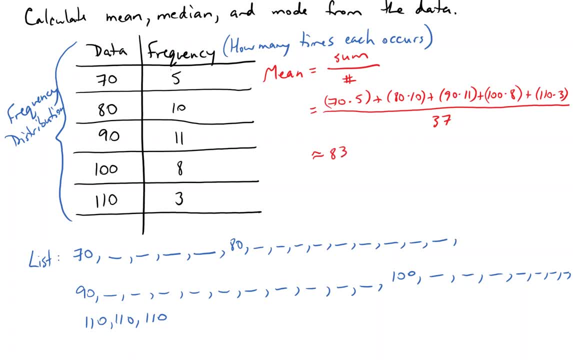 I typed it in real quick And I got approximately Approximately 88, 88.4 for the mean. Okay, All right, let's talk about the median. The median is simply the middle value. So where is the middle value? 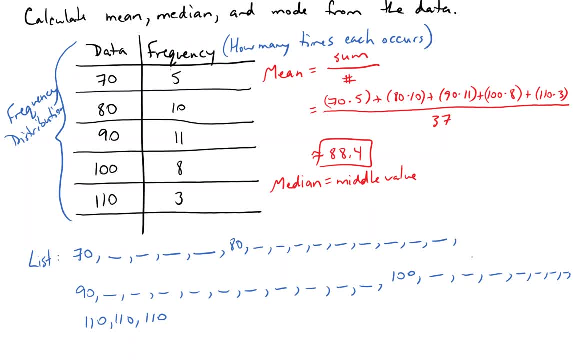 Well, there are 37 values here, And what I like to do is think of half of 37. Half of 37. Is a little bit more than 18.. So if I split this into two groups, then I'd have- if I have- 37 values. 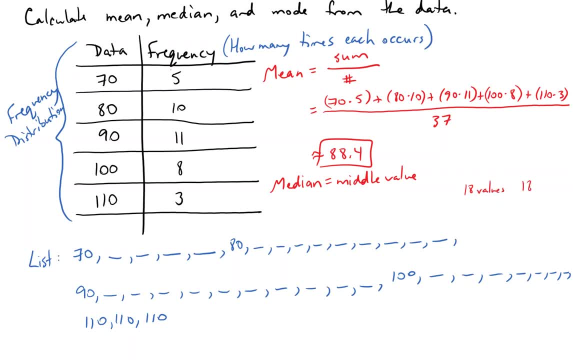 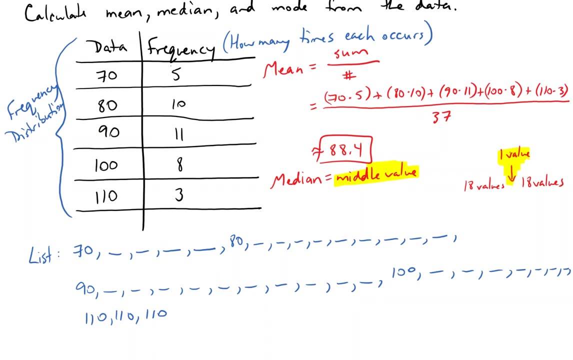 I'll have 18 values on one side, 18 values on the other, That's 36 values, And in the middle I'll have one value. So my median, my middle value will be this one value here, which happens to be the 19th value.